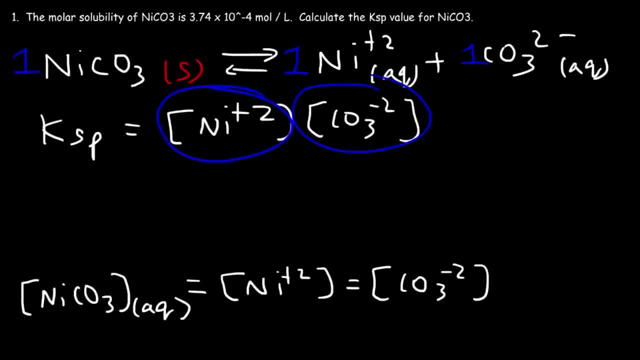 So in this example we just got to plug in the concentrations of nickel and carbonate, Which they're the same as this number. They're all equal to 3.7 times 10, to the negative 4.. So nickel is going to be the same number. 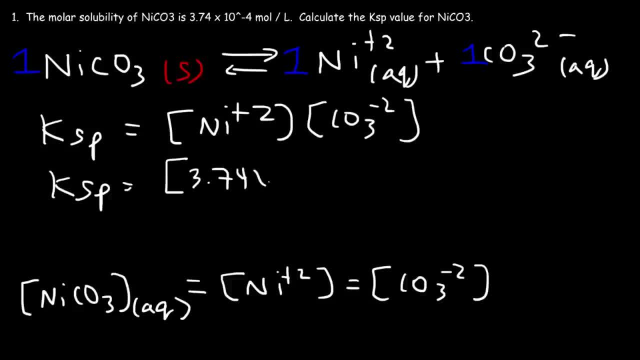 So nickel is going to be the same number And carbonate is also equal to the same value. So for this problem it's 3.74 times 10 to the negative 4 squared, And so the KSP for nickel carbonate is 1.4 times 10 to the minus 7.. 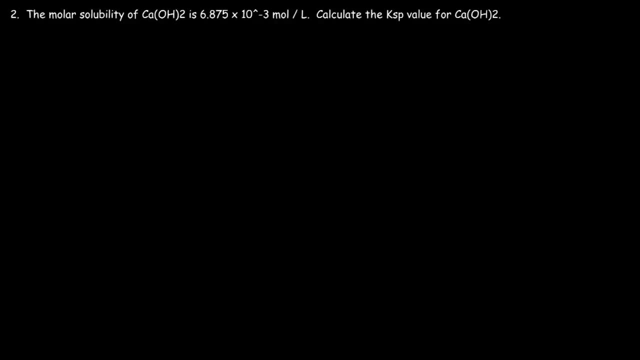 And therefore this is the answer. Now let's work on number two. The molar solubility of calcium hydroxide is 6.875 times 10 to the negative. 3. Calculate the Ksp value for calcium hydroxide. 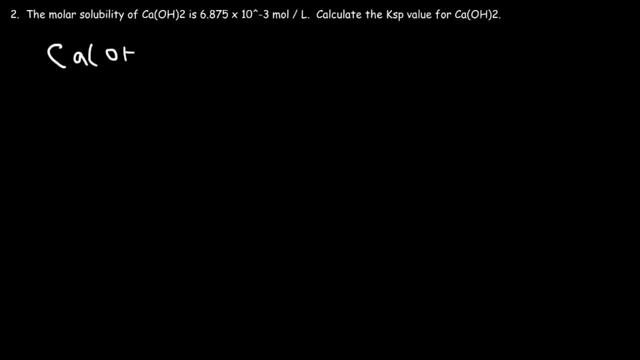 So first let's write the dissociation reaction. Solid calcium hydroxide dissociates into calcium and two hydroxide ions, And so these are in the aqueous phase. Now pay attention to the molar ratio. So we have a 1.. 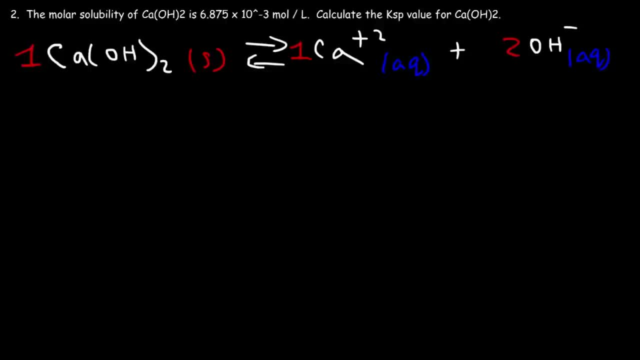 So, with this reaction, go ahead and calculate the Ksp value for this substance. Now let's calculate the concentrations of everything. The concentration of calcium hydroxide in the aqueous phase is given to us. That's the molar solubility. 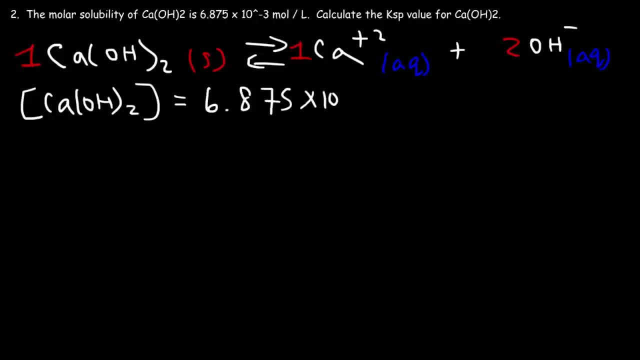 That's 6.875 times 10 to the minus 3.. Now the concentration of calcium. Notice that these two are in a one-to-one ratio, So therefore they have the same concentration. Now the concentration of hydroxide is going to be twice the concentration of this value, or twice the molar solubility, because there's a 2 here. 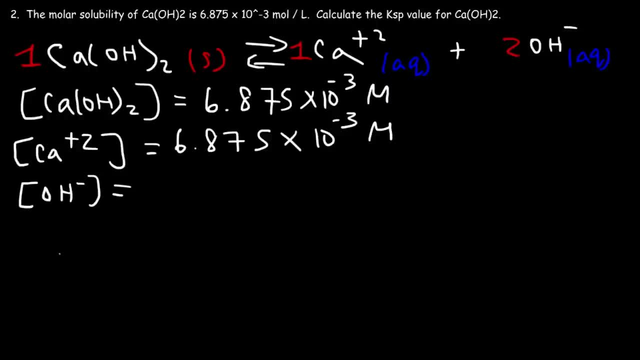 So, for those of you who want to show your work, here's what you can do. So, starting with calcium hydroxide, The molar concentration is 6.875 moles of CaOH2 per liter, So you can start with that. 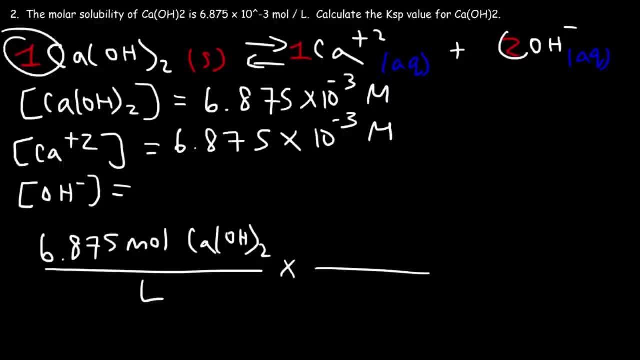 And then use the molar ratio. The molar ratio is 1 to 2.. So for every 1 mole of calcium hydroxide that dissolves, you could say that 2 moles of hydroxide ions are produced, And so you can cancel these units. 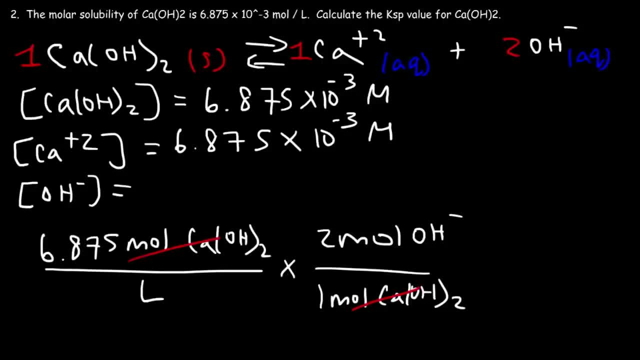 And now you have the concentration of hydroxide In moles per liter. So it's 6.875 times 10 to the minus 3, multiplied by 2. And so the concentration of hydroxide is 0.01375.. 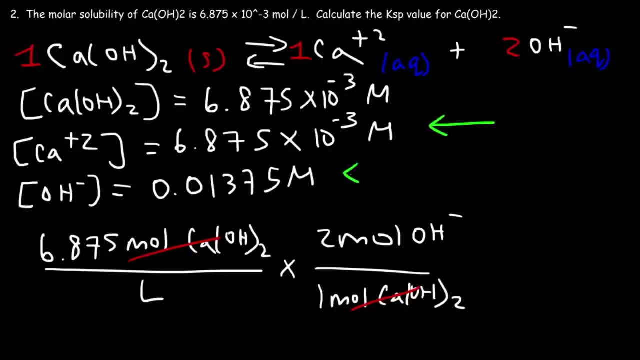 So now that we have the equilibrium concentrations of calcium and hydroxide, we can now calculate the Ksp value for it, And so Ksp based on this reaction is going to be equal to the calcium ion concentration multiplied by the hydroxide ion concentration. 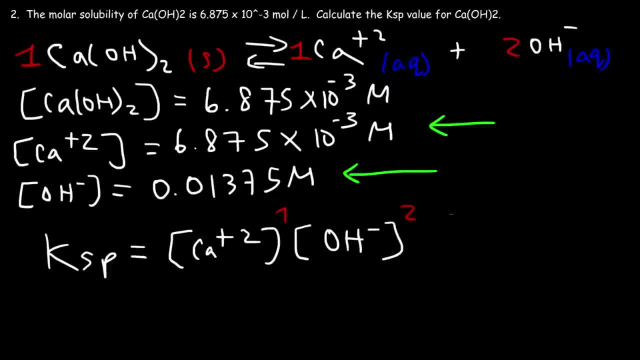 But that's going to be raised to the second power. Keep in mind, the coefficients turn into the exponents in the equilibrium expression, So now we just have to plug in the numbers that we have. So the concentration for calcium is 6.875 times 10 to the minus 3.. 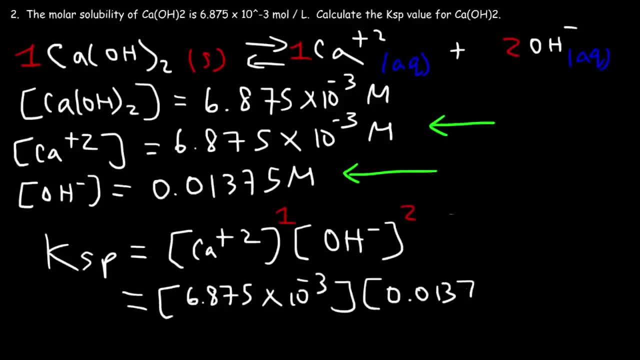 And for hydroxide it's 0.01375.. And we need to square it, And so this is equal to 1.3 times 10 to the negative 6.. So this is equal to 1.3 times 10 to the negative 6.. 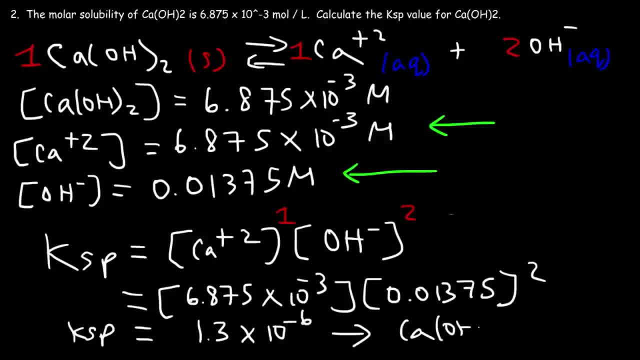 So this is equal to 1.3 times 10, to the negative 6.. So that is the Ksp value for calcium hydroxide. So now you know how to calculate the Ksp value, given the molar solubility. 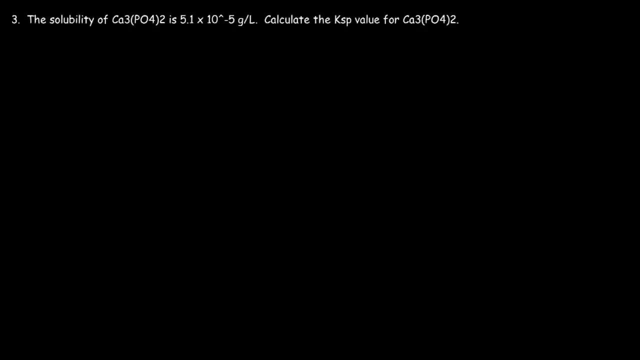 Number 3.. The solubility of calcium phosphate is 5.1 times 10 to the negative 5 grams per liter Calculate the Ksp value for calcium phosphate. So, like before, let's start out with a reaction. So we have solid calcium phosphate. 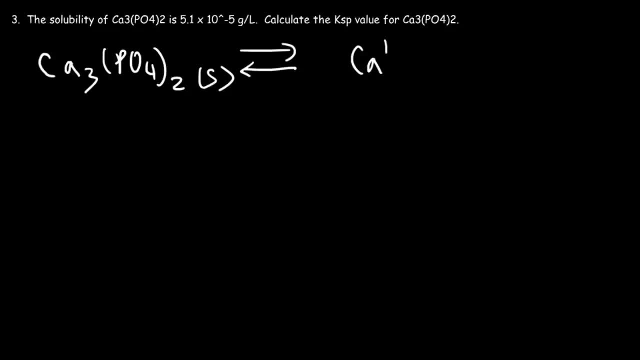 And it's going to ionize into the calcium plus 2 ion, which is in the aqueous phase, and also the phosphate ion. Now we need to balance the reaction. So notice that we have a subscript of 3 for calcium and a subscript for phosphate is a 2.. 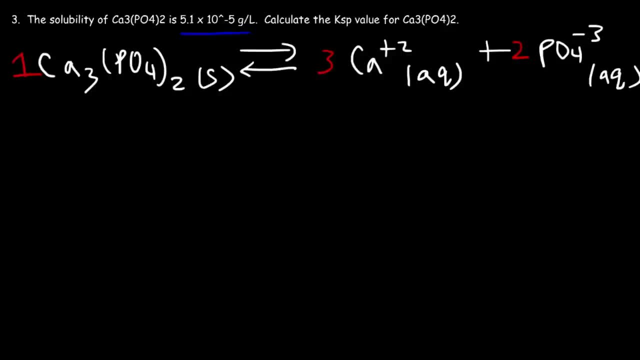 So now it's balanced And we're given the molar solubility in grams per liter as opposed to moles per liter. So the first thing we need to do is calculate the Ksp value, And we're going to calculate the molar solubility in moles per liter. 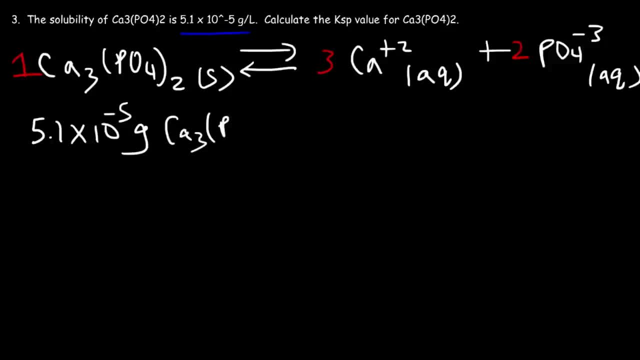 So let's start out with this. We need to find the molar mass of calcium phosphate. So let's go ahead and calculate it. The atomic mass of calcium is 40.08.. And there's 3 of them in this formula: unit. 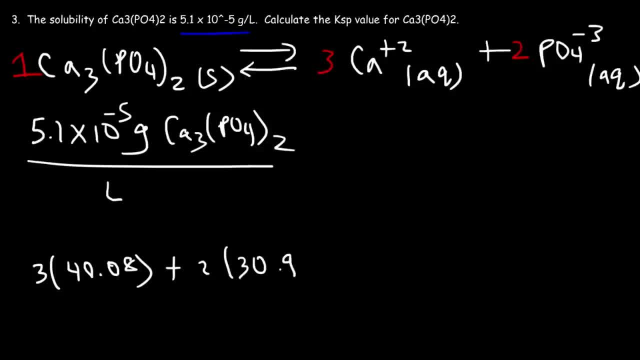 And then we have 2 phosphorus atoms, each with an atomic mass of 30.97.. And there's 8 oxygen atoms. So 3 times 40.08 plus 2 times 30.97 plus 8 times 16, that's equal to a molar mass of 310.18 grams per mole. 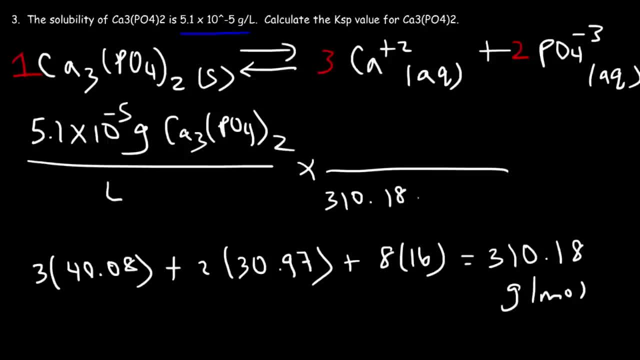 So we can say that there's 310.18 grams of calcium phosphate per 1 mole of calcium phosphate. So these units will cancel, And so it's going to be 5.1 times 10 to the minus 5, divided by the molar mass, which is 310.18.. 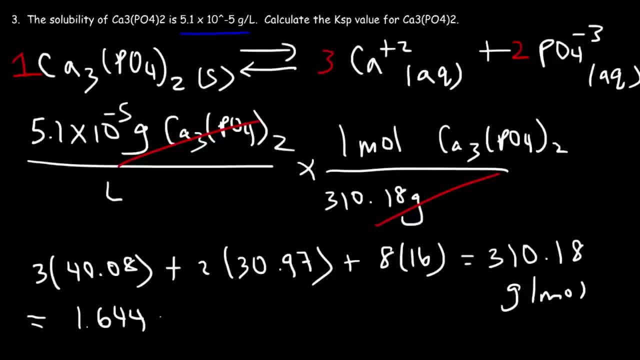 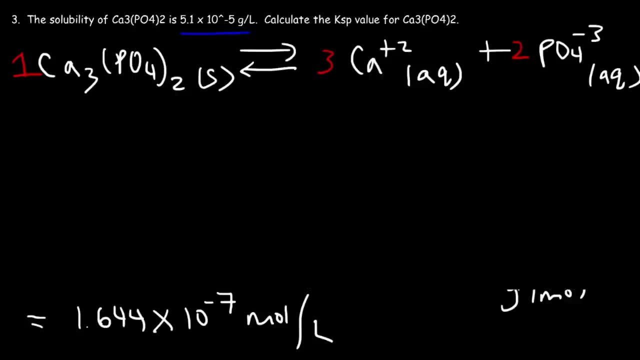 And so this is going to be 1.644 times 10 to the negative 7 moles per liter. So that's the molar solubility. That's the first thing we need to do before we calculate the Ksp. Now, keep in mind: this molar solubility represents the concentration of calcium phosphate that's dissolved in the solution. 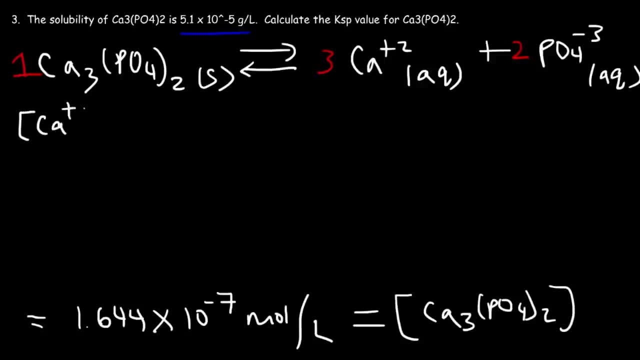 So now let's calculate the concentration of the calcium plus 2 ion. So notice that it's 3 times this particular value. So it's going to be 3 times 1.6.. 4.4 times 10 to the minus 7.. 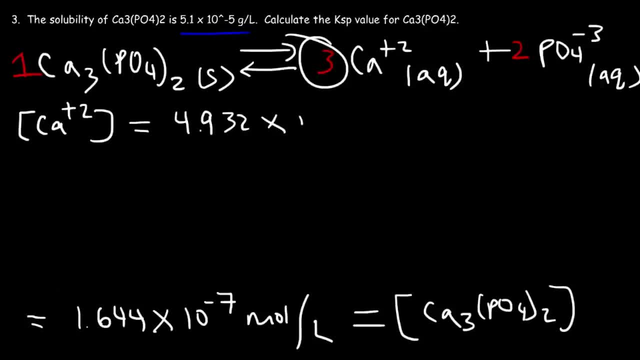 And so that's going to be 4.932 times 10 to the minus 7 moles per liter, or molarity Now, the phosphate ion concentration is simply twice the value. And keep in mind, if you want to show your work, you can write it like this: 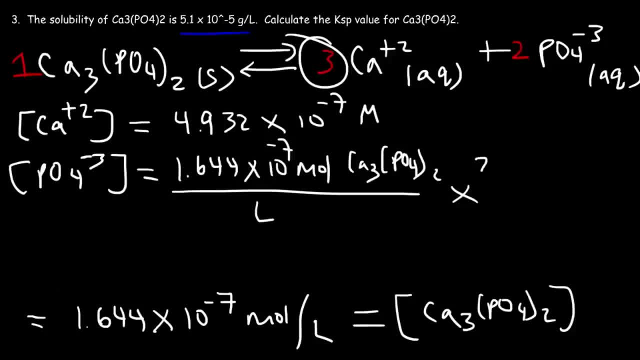 So you need to write that there's 2 moles of phosphate ions per 1 mole of calcium phosphate, And so that's why you need to multiply it by 2.. But for those of you who don't need to show your work for some reason, 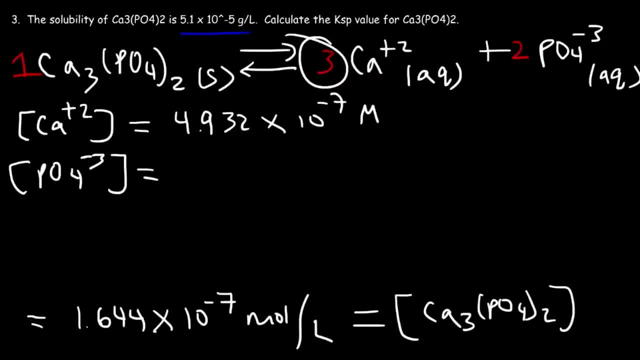 you can just multiply the molar solubility by 2, and then you'll get the phosphate ion concentration. So this is going to be 3.288 times 10 to the minus 7.. So now that we have the calcium and the phosphate ion concentrations at equilibrium, 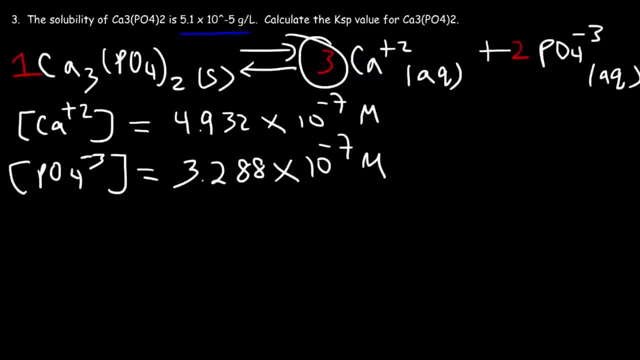 we can now calculate the Ksp value. Now, granted, the solubility that they give you is always the solubility at equilibrium. It's not the initial value. We don't need an ice table for this problem. So the Ksp value is 3.288 times 10 to the minus 7.. 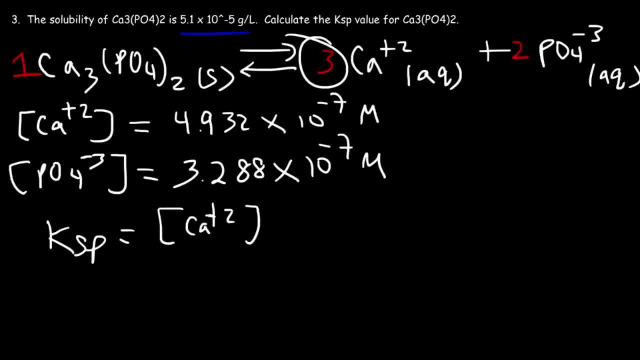 So the Ksp value is going to be the calcium plus 2 ion concentration raised to the 3rd power, since we have a coefficient of 3, and then times the phosphate ion concentration raised to the 2nd power. So the concentration of calcium, that's 4.932 times 10 to the negative 7.. 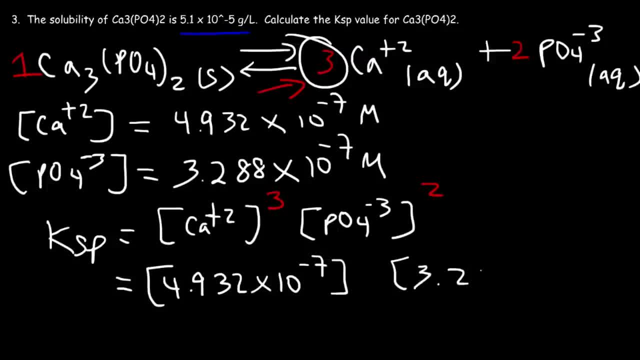 And for phosphate it's 3.288.. So the Ksp value is going to be 3.288 times 10 to the negative 7.. And don't forget to raise this to the 3rd power and that to the 2nd power. 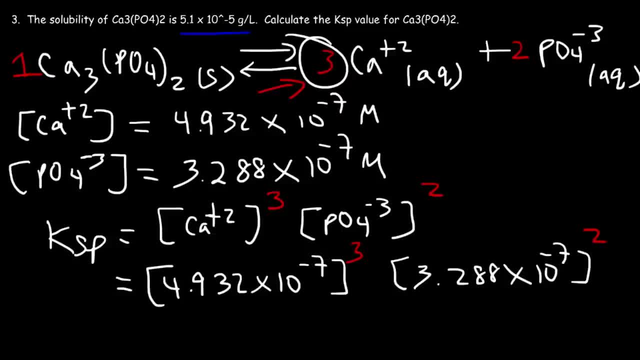 So go ahead and type in what you see in the calculator. So this is equal to 1.3 times 10 raised to the negative 32.. So this is the Ksp value For calcium phosphate. That's the answer Number 4.. 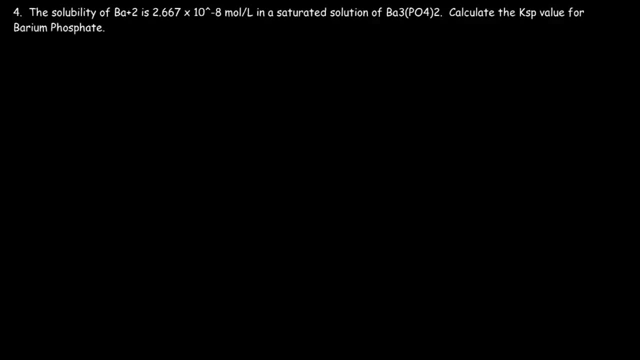 The solubility of the barium plus 2 ion is 2.667 times 10 to the negative 8 moles per liter in the saturated solution of barium phosphate. Calculate the Ksp value for barium phosphate. So first let's write the dissolution reaction. 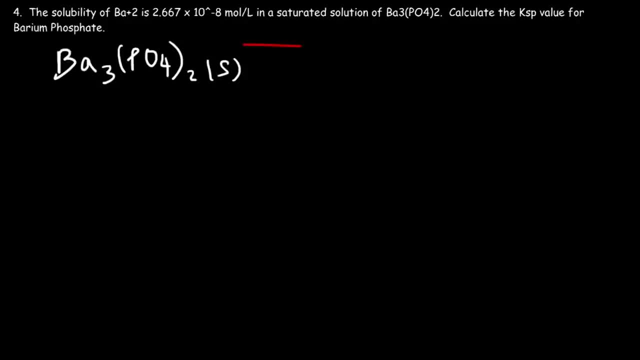 Solid barium phosphate. It's going to ionize and form the barium plus 2 ion and also the phosphate ion And looking at the subscripts, it's 3 and 2.. So to balance it, we're going to use a 1 on the left, a 3 in front of barium and a 2. 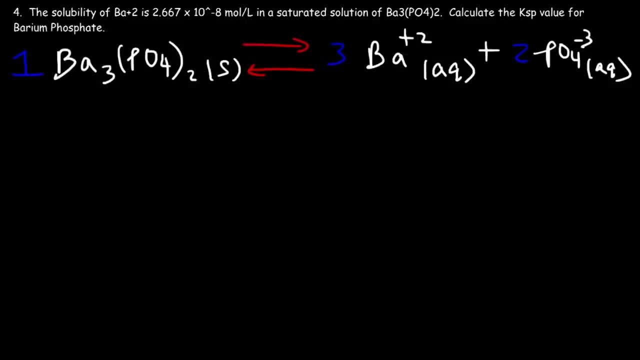 in front of the phosphate ion. Now we need to calculate the equilibrium concentrations. So we're going to use a 1 on the left, a 3 in front of barium and a 2 in front of phosphate ion. So we're going to calculate the equilibrium concentrations of these two ions. 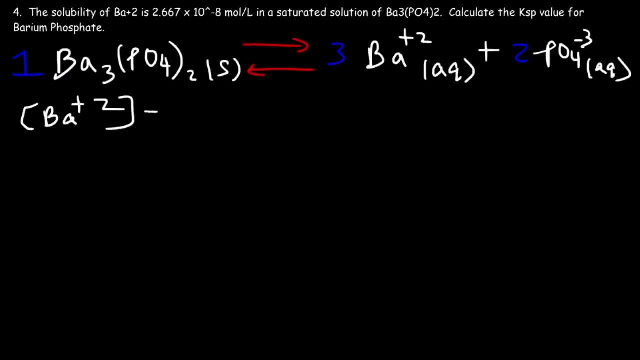 We already have barium plus 2, which is good. The concentration for that is 2.667 times 10 to the minus 8. And that's in the saturated solution. so that's the equilibrium concentration. So what we need to do is take this value and convert it to the concentration of phosphate. 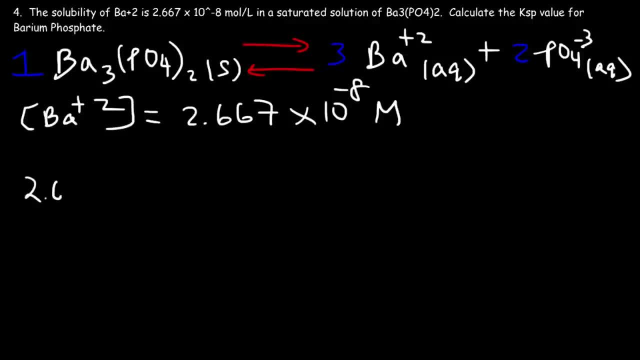 And we can use the balanced chemical equation to do that. So let's start with 2.667.. And we're going to use the balanced chemical equation to do that, So let's start with 2.667 times 10 to the minus 8 moles of Ba, plus 2 per liter. 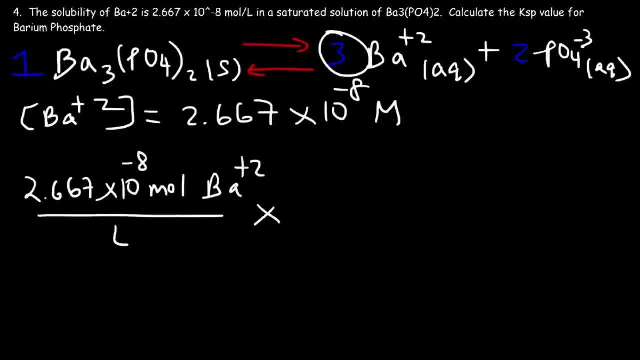 And the molar ratio is 3 to 2.. So for every 3 moles of barium that dissolves, 2 moles of phosphate will dissolve along with it. So we could cancel these two units. So it's going to be 2.667 times 10 to the minus 8.. And we're going to use the balanced chemical equation to do that. So let's start with 2.667 times 10 to the minus 8.. So it's going to be 2: 2 division by 5 times 8 minus 1 over 3 minus 1.. 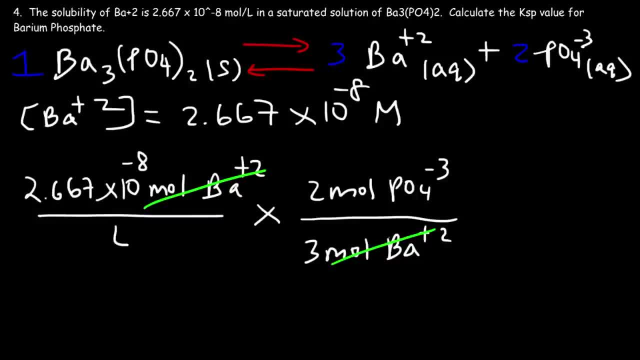 You get 2 x 10 to the minus 8, multiplied by 2, And so the phosphate ion concentration in this problem is 1.778 times 10, raised to negative 8.. Now let's calculate the Ksb. 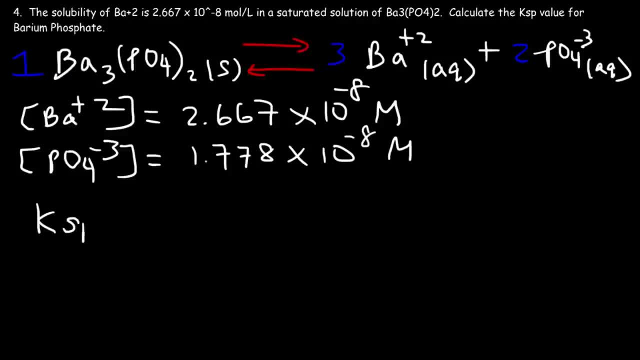 So let's write the equilibrium expression to our formula. So here we have just 1.778 times 10 to the minus 8. expression: it's going to equal the barium plus two concentration times the phosphate concentration. and we need to raise this to the third power and the. 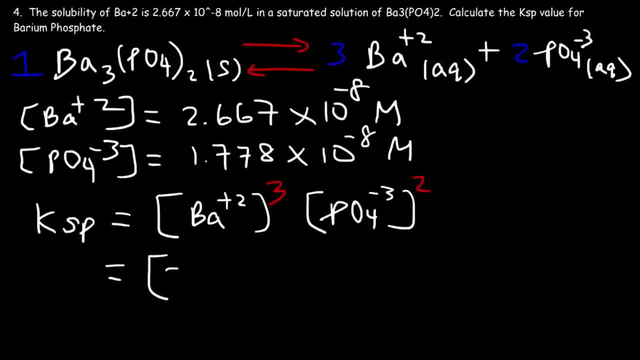 phosphate concentration to the second power. so it's going to be two point six, six, seven times ten to the minus eight raised to the third power, and then one point seven, seven, eight times ten to the minus eight raised to the second power. so the answer that I got for this problem is five point nine nine seven. 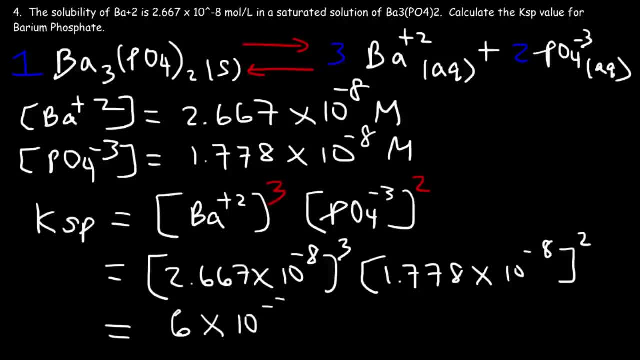 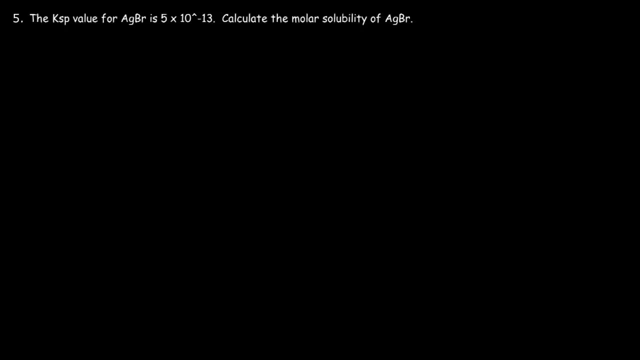 which is basically six times 10 to negative 39. so that's the KSP value for barium phosphate in this problem, and so this is the answer. now let's work on a different type of problem. so we have the KSP value for a GPR. what is the molar solubility of? 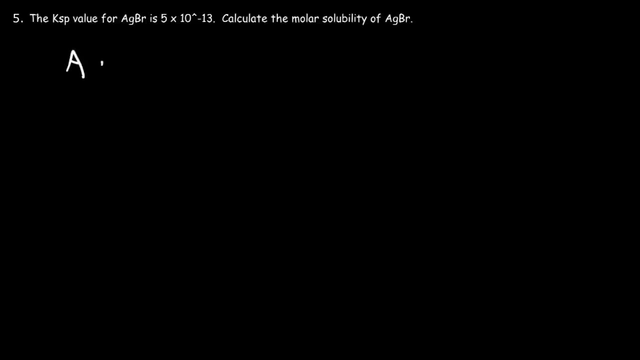 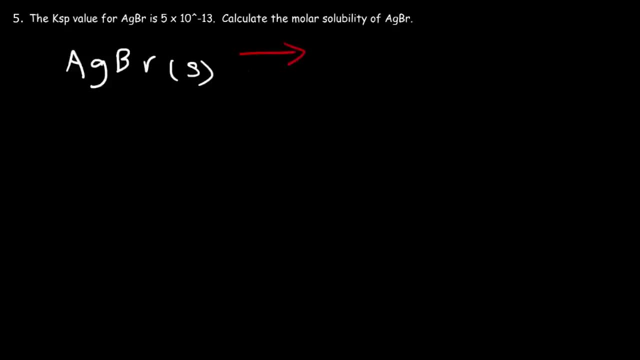 write the dissolution reaction for a GPR. so if you were to put solid silver bromide in water, some of it will dissociate into silver cations and bromide anions. now let's make an ice table. initially, the concentration of AG and BR will be zero. as a result, the reaction has to shift to the right. so 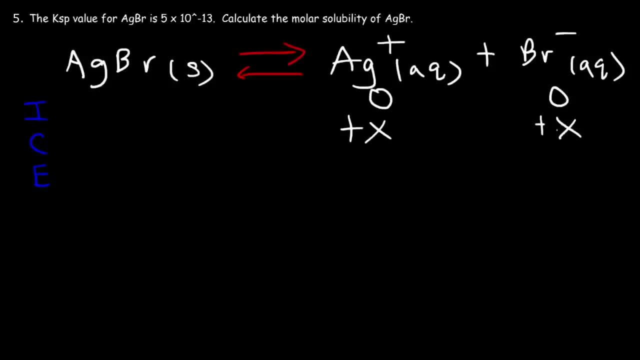 therefore, the products will increase by X. the molar ratio is one-to-one. now to write the equilibrium expression for this reaction, it's going to be products divided by the reactants. so the products are AG plus and BR minus. the reactant is a GPR. however, you cannot include any. 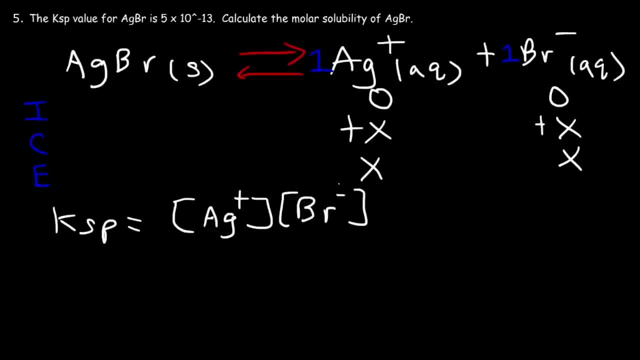 liquids or solids in the equilibrium expression. so this is the KSP expression for this example. this example now KSP for a GPR is five times 10 to the minus 13. the concentration of AG plus is X and for bromide is X as well. so X times X is X. 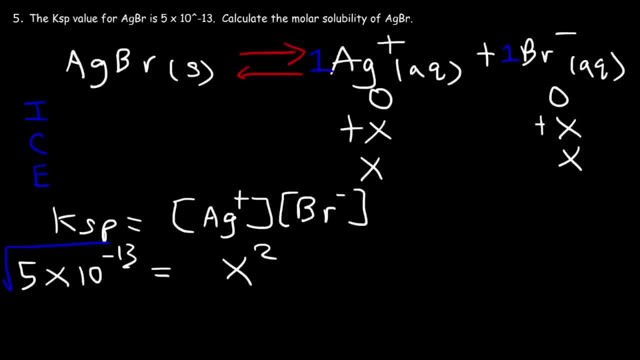 squared. now let's take the square root of both sides. so X is equal to seven point zero, seven times 10 to negative seven moles per liter. notice that X represents the concentration of AG plus and BR minus. now notice that everything is in a one-to-one ratio. so therefore the concentration of silver bromide that 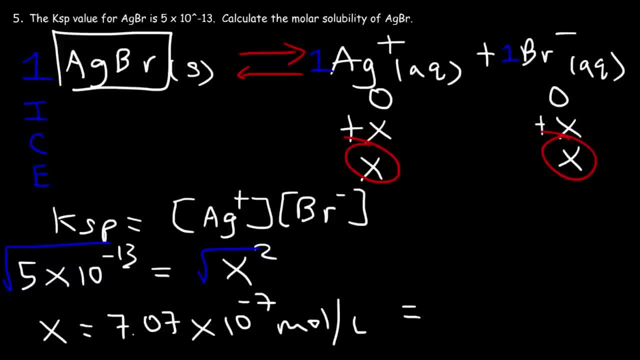 is dissolved in a solution. some of it may be in a solid phase, but the amount that's dissolved in a solution is equal to the concentration of AG plus and BR- due to the one to one molar ratio. so X is also equal to the concentration of the. 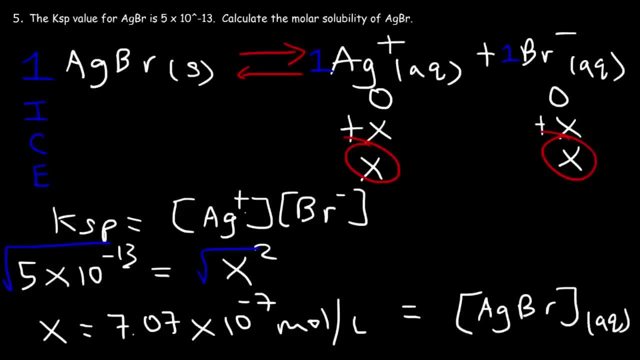 dissolved silver bromide in the solution. so anytime you want to find or calculate the molar solubility of the solid product, the portion that's dissolved in the solution, all you need to do is calculate X. X represents the molar solubility of the substance, and so this is the answer. seven point zero, seven. 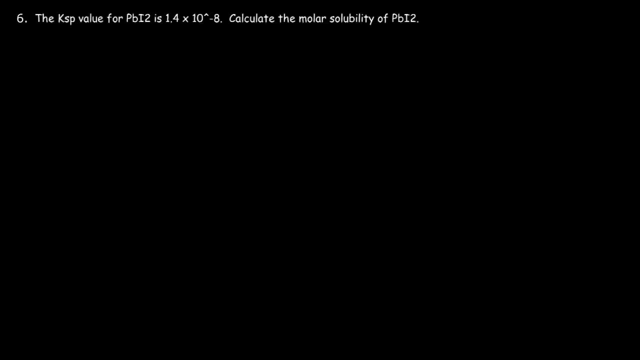 times ten to the minus seven moles per liter. For the sake of practice, let's try another one. You can work on this example if you want to So calculate the molar solubility of lead iodide or lead 2 iodide. So all we need. 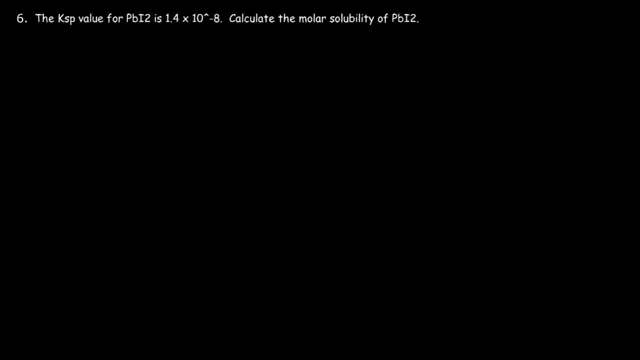 to do is calculate the value of X. That's going to be the concentration or the solubility of lead iodide that's actually dissolved in a solution. So let's start with the substance in its solid form and then it's going to dissociate into Pb plus 2 and also iodide. 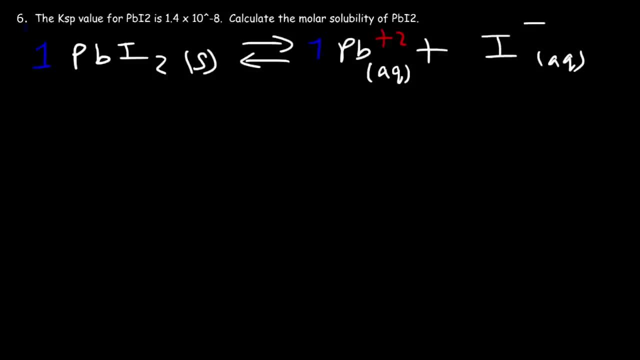 Now we need to balance the reaction. So this is going to be 1 and this is going to be 2.. Now let's make an ICE table. So this is going to be 0 and 0.. Now this is going to increase by 1x and this is going to increase by 2x, based on the molar ratio. 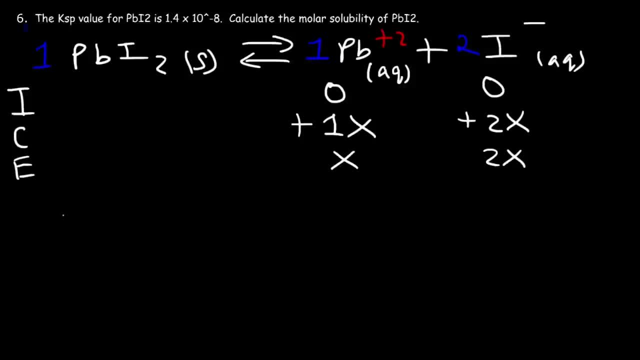 that you see there. So now let's write the KSB expression for this reaction. So it's going to be Pb plus 2 and then times the concentration of iodide. Now the coefficients will turn into the exponents in the equilibrium expression. Now KSB for lead. 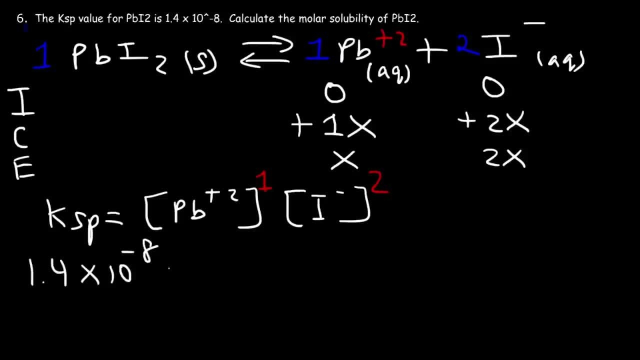 2, iodide is 1.4 times 10 to negative 8 and lead plus 2 is equal to X and iodide is equal to 2x. 2x times 2x is 4x squared And X times 4x squared is 4x cubed. So 1.4 times 10 to the negative 8 is equal to. 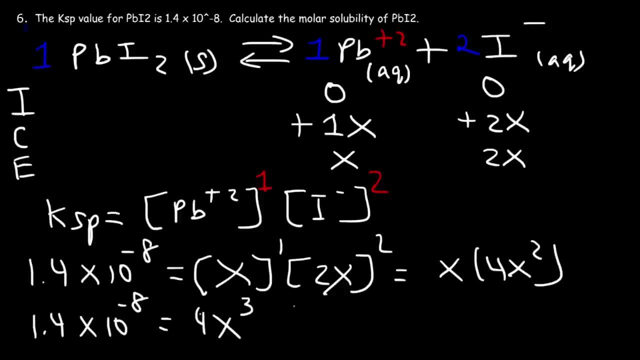 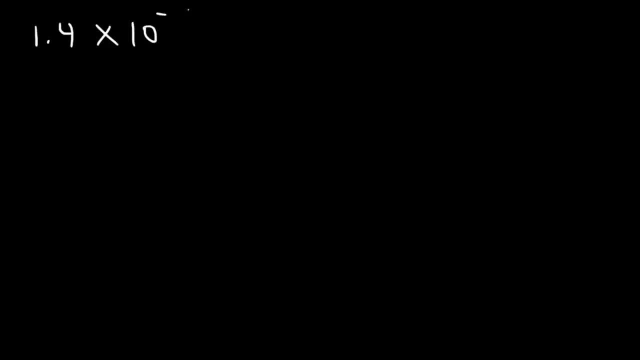 4x cubed. And keep in mind our goal is simply to calculate the value of X. So let me rewrite this on top. So at this point, it's all algebra. So what I'm going to do is I'm going to divide both sides by 4, initially. 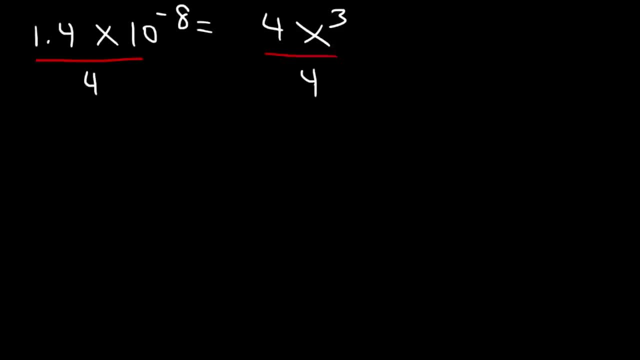 1.4 times 10 to the negative. 8. divided by 4, that's 3.5 times 10 to the negative 9.. And that's equal to X cube. Now the next thing that you want to do is you want to. 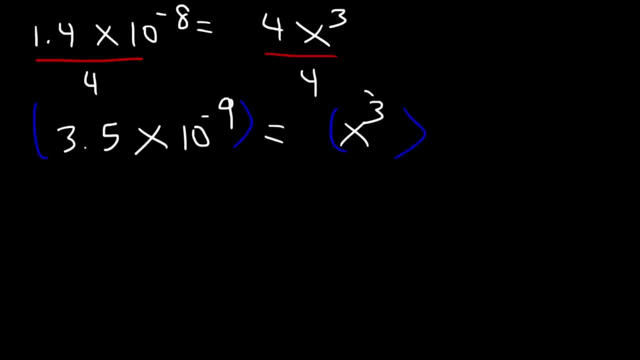 raise both sides to the 1 third power based on the number you see here. So raise it to the reciprocal of that value. When you raise one exponent to another, you need to multiply 3 times 1 third. 3 over 3, that's. 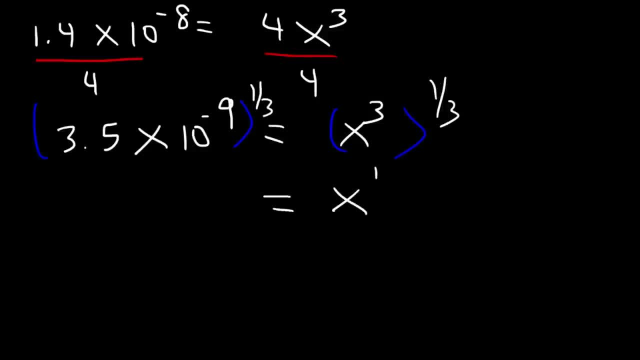 one the threes cancel. to get X to the first, power is simply X. so it's 3.5 times 10 to the negative 9 raised to the 1, 3rd, or you could take the cube root of it, and so X is 1.5, 2 times 10 to the minus 3 moles per liter or molarity, and 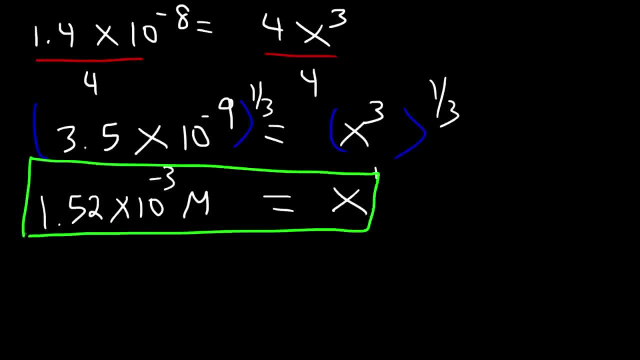 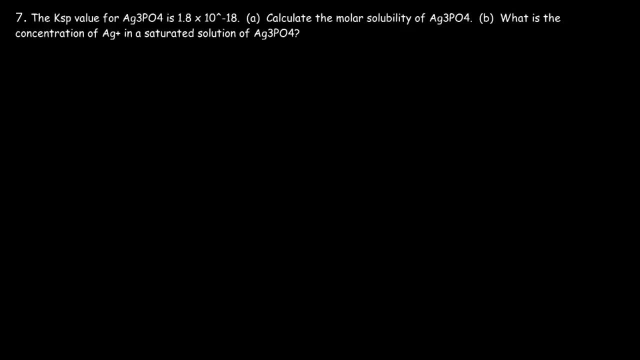 that's the molar solubility of lead to iodide. you just got to calculate the value of X. the KSP value for silver phosphate is 1.8 times 10, raised to the negative 18. calculate the molar solubility of a g3 peel for. so this is: 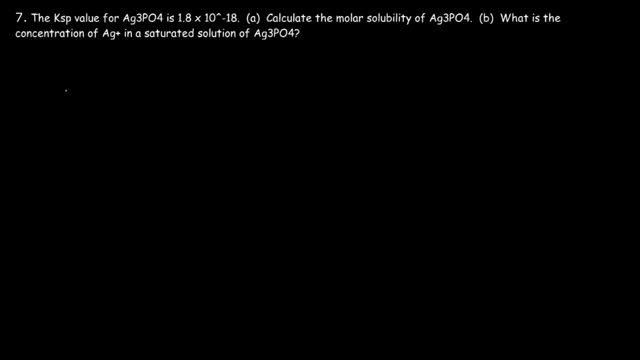 similar to the first two problems. go ahead and try this. so let's begin with the reaction. so we have a g3 peel for in the solid phase and then it's going to dissociate into you a g plus, which is in the aqueous phase, and also phosphate, which is also 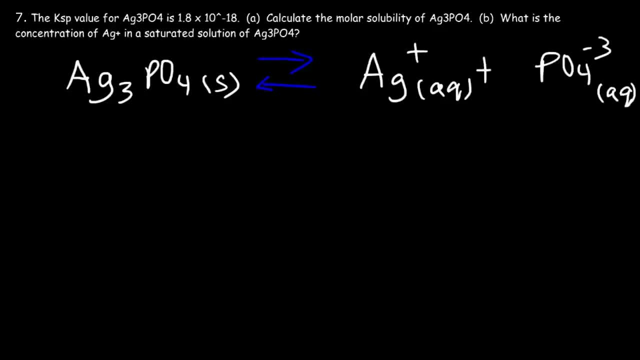 in a aqueous phase. now let's go ahead and balance the reaction. so notice that the subscript history will put it 3 in front of 80 plus 1 in front of peel. for now let's make a nice table, so this is not be 00. 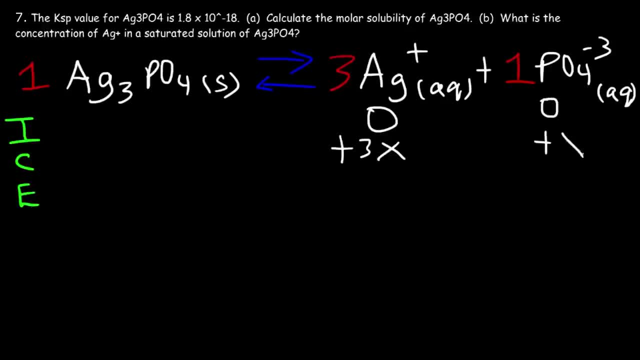 0, 0, 0, 0, 0 plus 3x plus x, and then 3x and x. So the KSP expression is going to be Ag plus times phosphate. And then we need to raise this to the third power and this to the first power. 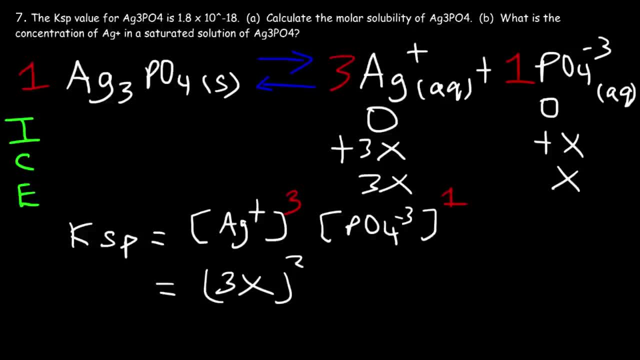 Now, Ag is equal to 3x, and that's raised to the third power. Phosphate is equal to x, 3 to the third power is 27.. So this is 27x cubed times x, And so this is 27x to the fourth. 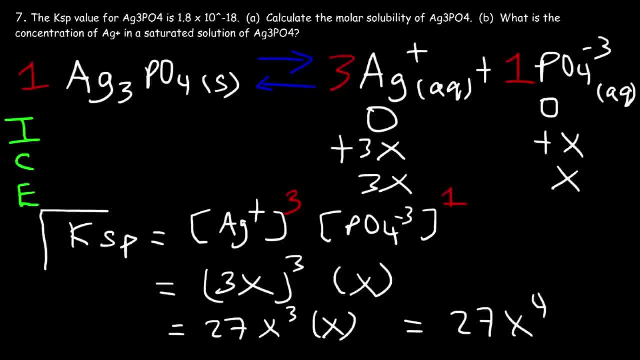 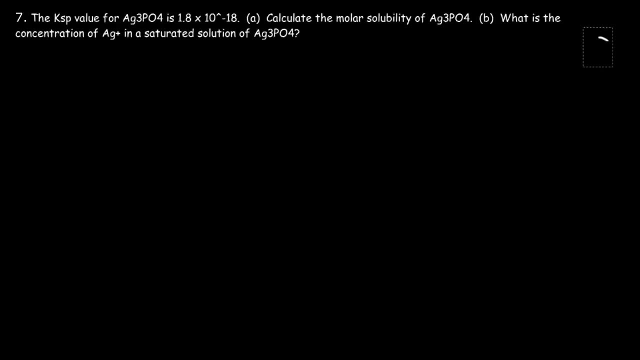 Now I'm going to show you a shortcut method that can help you to get this expression- The fact that KSP is equal to 27x to the fourth- And then we'll come back to this problem. Now let's start with our first example, which was AgBr. In this substance, notice that the 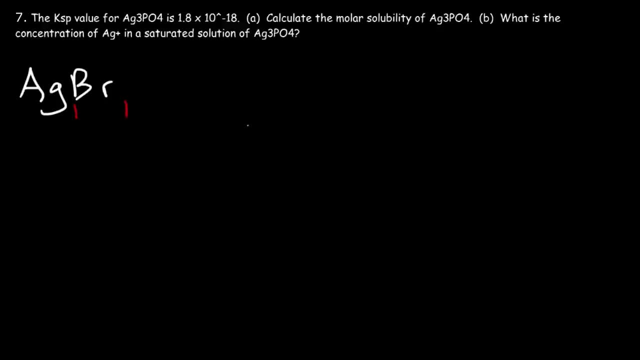 subscripts is 1 and 1.. So to calculate, the KSP for Ag is going to be 1x raised to the first power and for Br, 1x raised to the first power. So you get this expression: The KSP is equal to x squared. 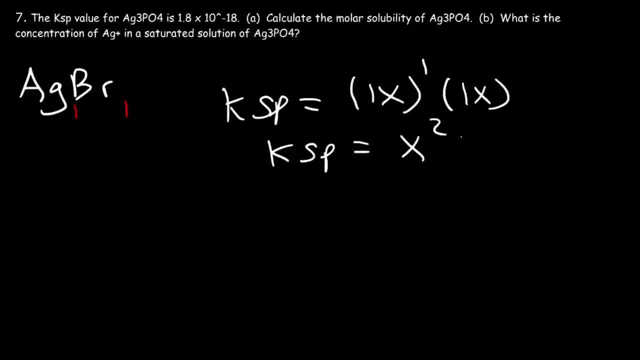 And if you need to calculate the molar solubility, just simply calculate x. Now for the second example. it was PbI2 or Pb1I2.. So to calculate the KSP expression for Pb, it's going to be 1x raised to the first power. 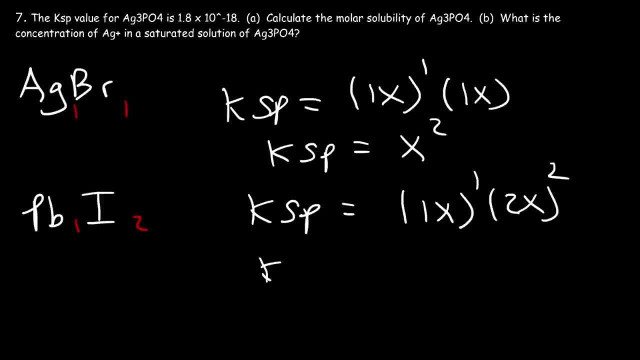 For I2, 2x raised to the second power, And this gave us this expression: KSP is equal to 4x cubed. So now for our third example. This works if you're not dealing with the common ion problems, by the way. 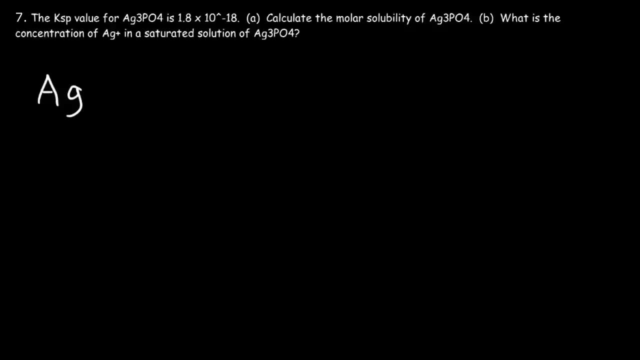 If you have a common ion problem- which I'll cover that in another video- you need to actually write out the ICE table. But for a problem like this, if you're given the KSP value and you want to calculate the molar solubility and there's nothing else given to you, 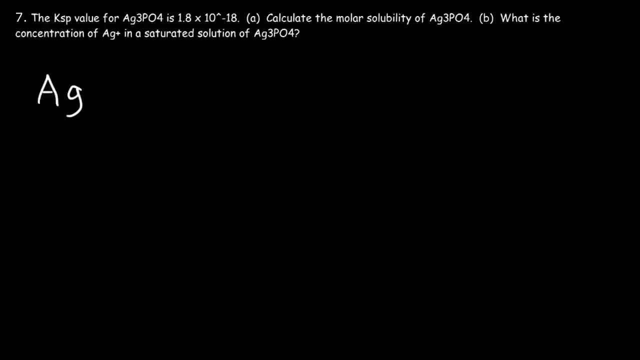 then you could use this technique. So I just want to highlight that fact. So, for this example, we had Ag3PO4.. The subscript for PO4 is a 1, because nothing was there. So the KSP is going to be 1x raised to the first power. So this is going to be 1x raised to the first power. So for this example, we had Ag3PO4.. The subscript for PO4 is a 1, because nothing was there. So the KSP is going to be 1x raised to the first power. 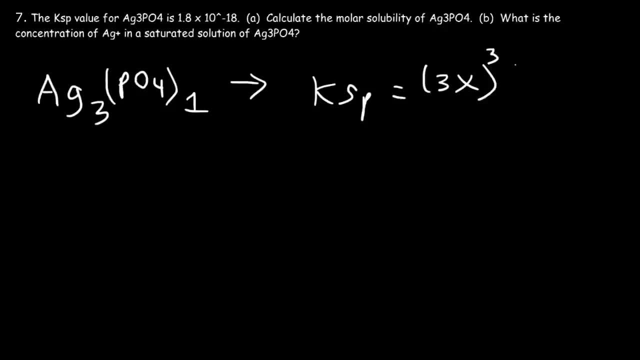 So this is going to be: for Ag, it's going to be 3x raised to the third power, And for phosphate, 1x raised to the first power. And so this is going to be 27x cubed multiplied by x. 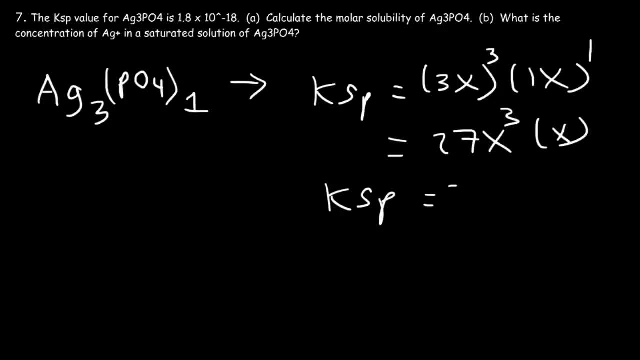 And so that's how we got the expression. KSP is 27x to the fourth, So now let's go ahead and finish this problem. So the KSP for silver phosphate is 1.8 times 10, raised to negative 18.. 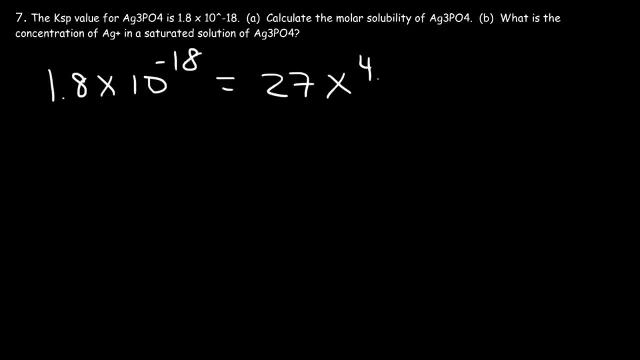 And that's equal to 27x to the fourth power. Now the first thing we're going to do is divide by the coefficient 27.. That's step one. So if you divide it by 27,, this is going to be 6.67 times 10 to the negative 20.. 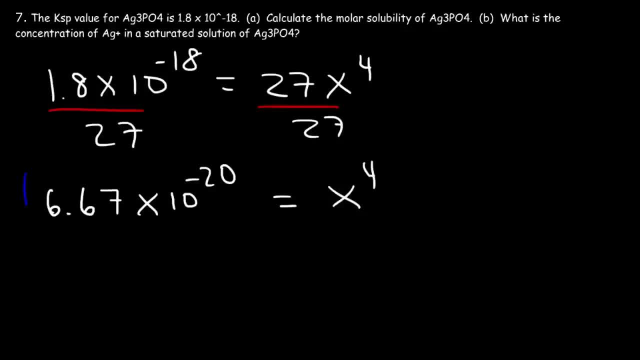 And that's equal to x to the fourth. Now, last time we raised everything to the one-third, This time because there's a 4, you want to raise everything to the one-fourth power, Because 4 times one-fourth is 1.. 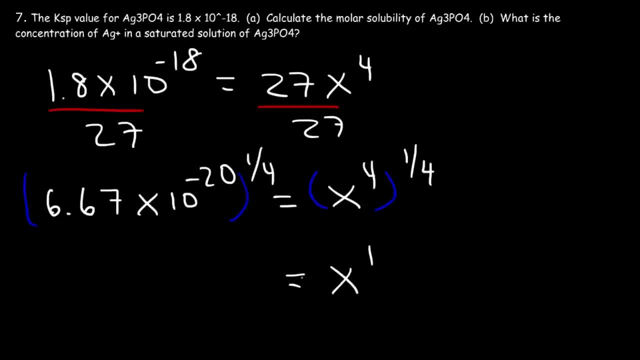 So you want to take the fourth root of 6.67 times 10 to the negative 20.. And so the molar solubility is 1.607 times 10 to the negative 5.. You can write more, You can write a molarity, or you can say moles per liter. 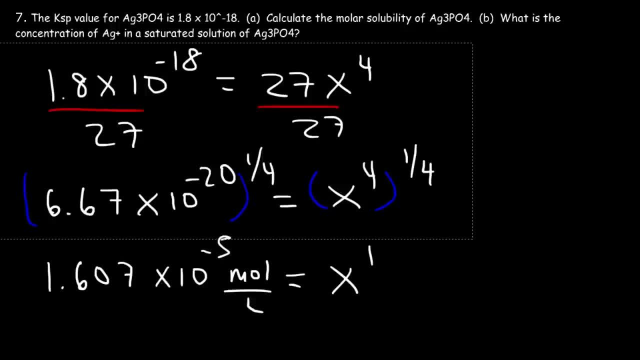 So that's the molar solubility of silver phosphate. Now let's move on to part B: What is the concentration of Ag plus in a saturated solution of silver phosphate? So how can we find the answer? I'm going to rewrite the reaction that we had in the beginning. 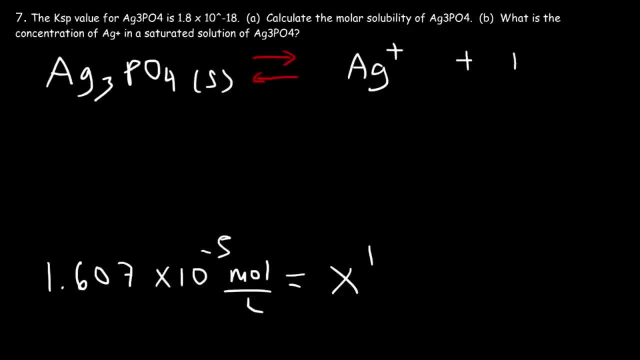 So this was 3, and this was 1.. Now keep in mind: x is the molar solubility for this substance, For Ag3PO4.. So that's how much silver phosphate is dissolved in a solution, in a saturated solution. 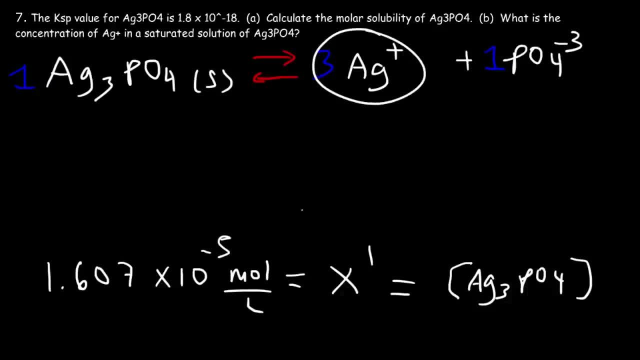 So what we need to do is convert it to this value. Notice that the ratio is 1.2.. So we simply have to multiply our answer by 3.. But if you want to show your work, here's what you can do. 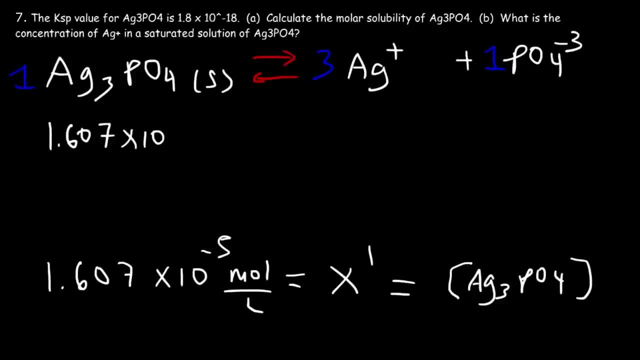 So start with what you have: 1.6 times 10 to the negative 5 moles of silver phosphate That's dissolved in a solution per liter. And now, for every mole of Ag3PO4 that's dissolved, there's going to be 3 moles of Ag plus dissolved along with it. 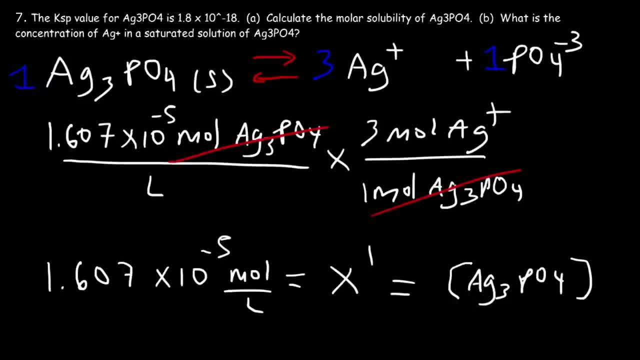 And so that's why we need to multiply it by 3.. So now we're going to have moles over liters for Ag plus. So the concentration of Ag plus in a saturated solution of silver phosphate is going to be 4.821 times 10, to the negative 5.. 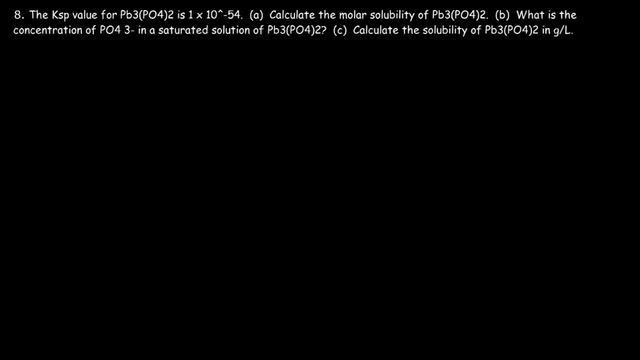 And so that's the answer. The Ksp value for lead phosphate is 1 times 10 to negative 54.. Calculate the molar solubility of Pb3PO4 to lead 2 phosphate. So let's use the shortcut method. 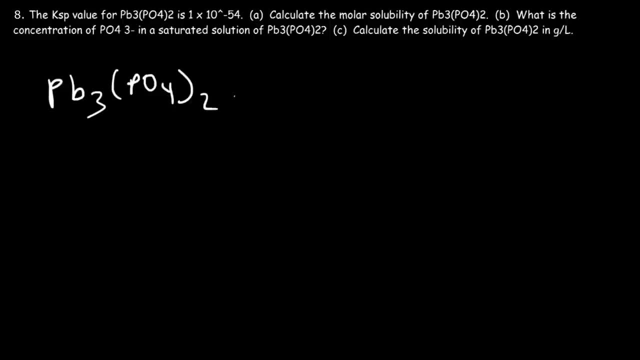 Let's write an equation that relates Ksp to x. So notice that the subscript for lead is 3, so it's going to be 3x to the 3rd power, And for phosphate it's 2, so it's going to be 2x raised to the 2nd power. 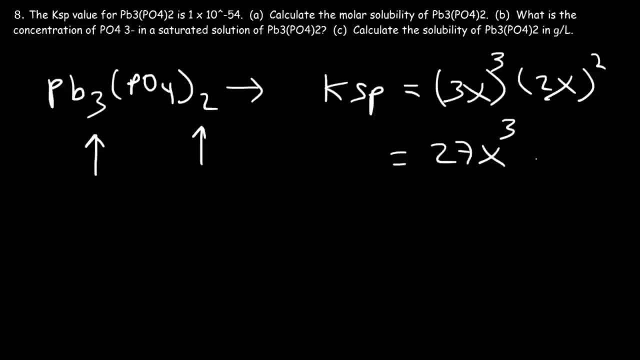 3 to the 3rd is 27.. And 2 squared is 4.. 27 times 4 is 108. So Ksp is equal to 108 times x to the 5th power. So let's replace Ksp with 1 times 10 to the negative 54.. 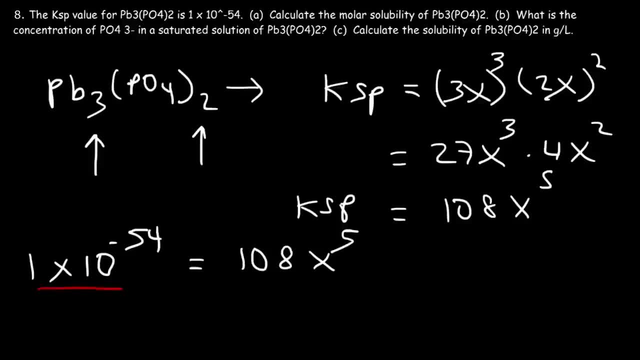 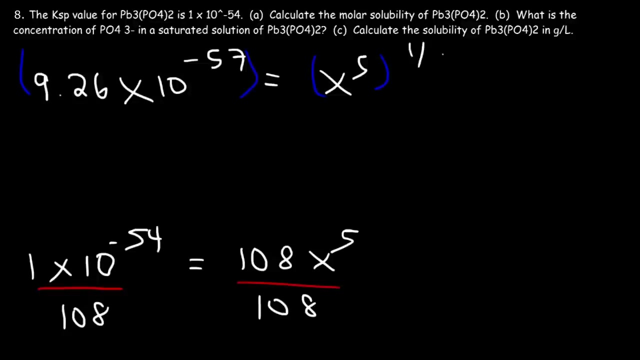 And so let's start by dividing both sides by 108.. So it's going to be 9.26 times 10, to the negative 57. And that's equal to x raised to the 5th power. So we need to raise both sides to 1 over 5.. 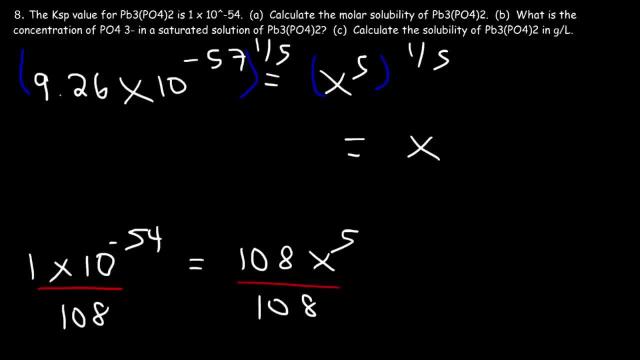 So on the right side this is going to equal x. On the left side this is going to be 6.21 times 10 to the negative 12 moles per liter. And so that's That's the answer for Part A. 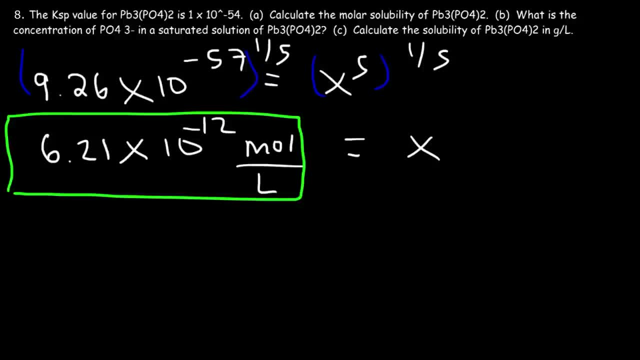 Now let's move on to Part B. What is the concentration of phosphate in a saturated solution of lead-2-phosphate? So let's write the reaction first. So lead-2-phosphate is going to associate into the Pb plus 2 ion and also the phosphate ion. 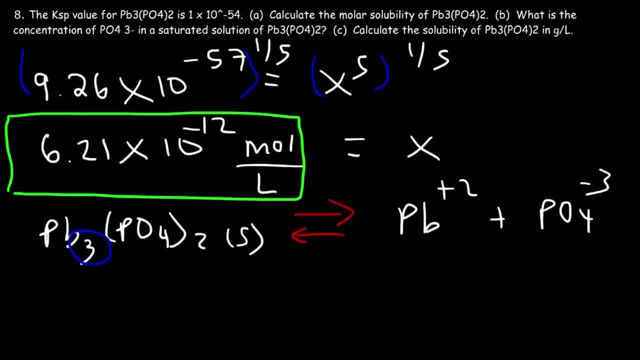 Now the coefficients- I mean the subscripts, are 3 and 2. So to balance it, we need to put a 3 here and a 2 in front of phosphate. So to calculate the concentration of phosphate, notice that it's twice the value of the amount of lead-2-phosphate dissolved in the solution. 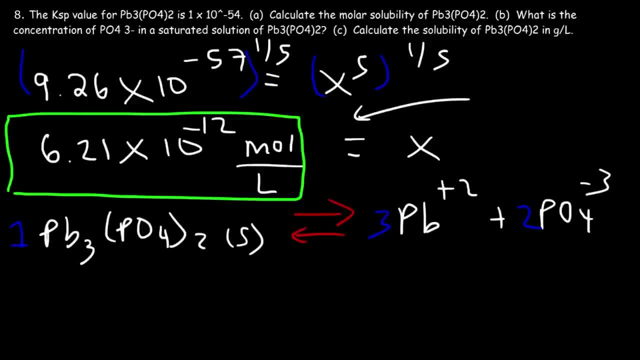 It's a 1 to 2 ratio. So if this represents the solubility of this substance, then the concentration of phosphate is simply going to be this number multiplied by 2.. So it's going to be 6.21 times 10, to the negative, 12 times 2.. 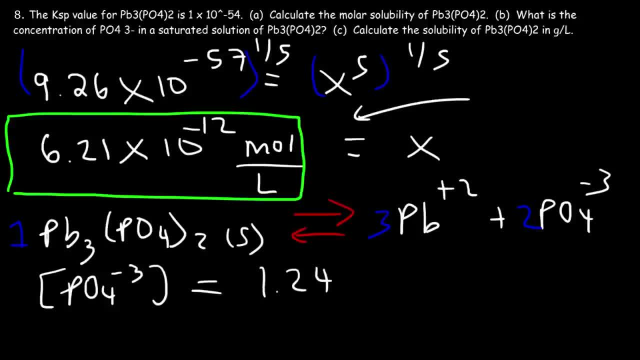 And so the phosphate concentration is 1.242 times 10 to the negative 11.. And so that's it. So let's say, if we need to calculate the lead-2-ion concentration, for example, Notice that the molar ratio is 1 to 3.. 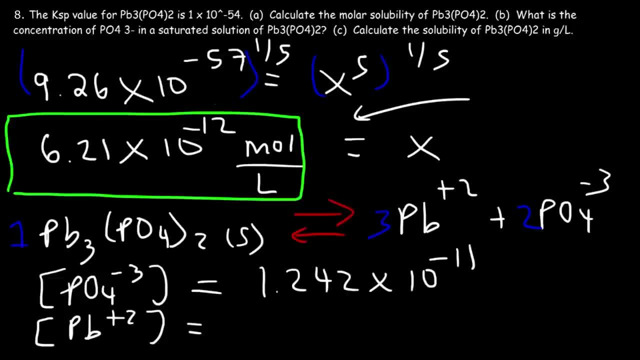 So it's going to be 3 times this number. So 6.21 times 10 to the negative 12, multiplied by 3. So that's going to be 1.863 times 10 to the minus 11.. So once you have the molar solubility, 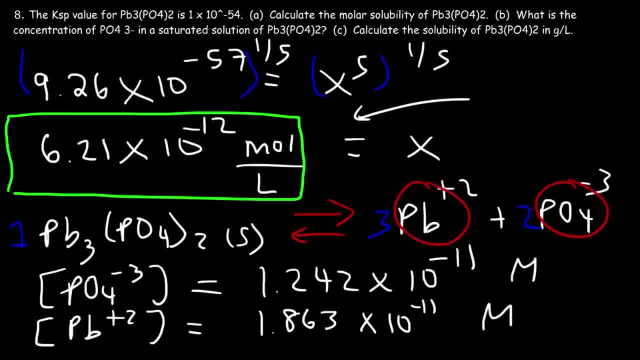 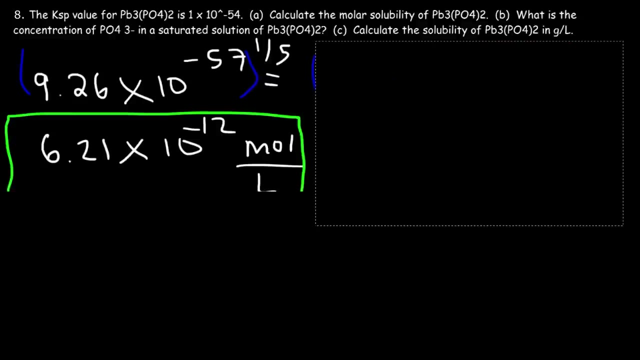 you can easily calculate the concentration of any product ion just by multiplying by the coefficient that you see here. Now let's move on to Part C: Calculate the solubility of lead-3-phosphate in grams per liter. So we're going to start with this number. 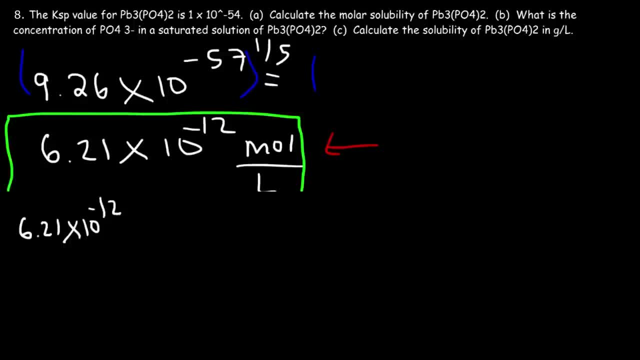 6.21 times 10 to the minus 11.. Minus 12 moles of lead-3-phosphate per liter, And all we need to do is convert moles into grams. So we need to calculate the molar mass of lead-2-phosphate. 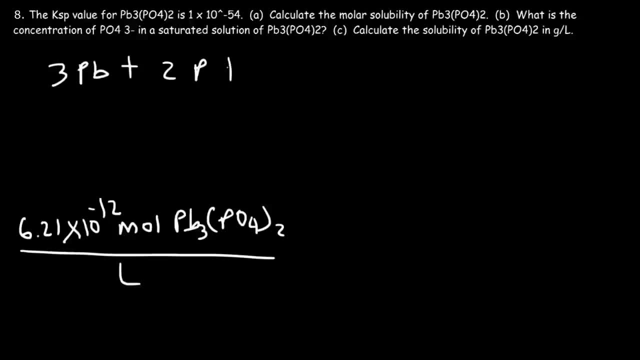 So there's 3 lead atoms, 2 phosphorus atoms and 8 oxygen atoms. Now the molar mass of lead is 207.2.. For phosphate it's 207.2.. For phosphorus it's 30.97.. 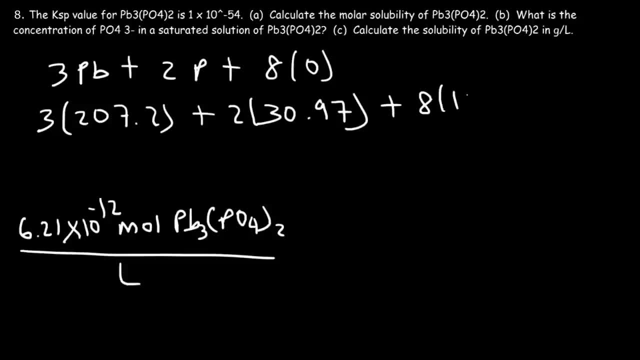 And for oxygen it's 8 times 16.. So let's go ahead and plug in these numbers. So this is 811.54 grams per mole. So we're going to put 1 mole on the bottom, That's 1 mole of Pb3PO4.. 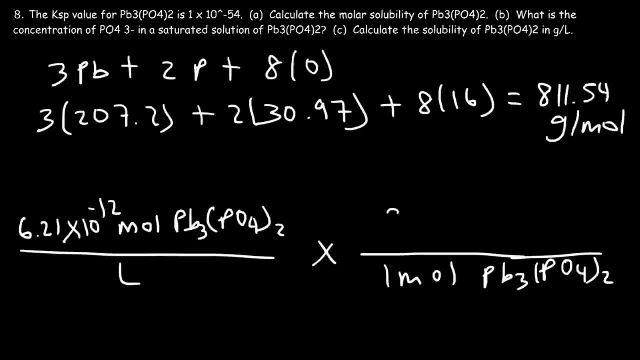 And it has a mass of 811.54 grams. So the unit's moles of lead-phosphate will cancel, And so this will give us the solubility in grams per liter. So it's going to be 6.21 times 10 to the negative 12.. 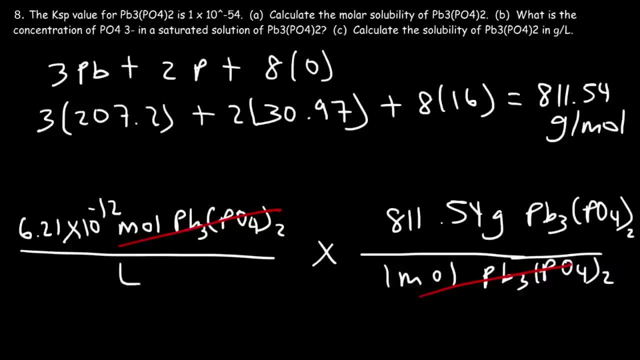 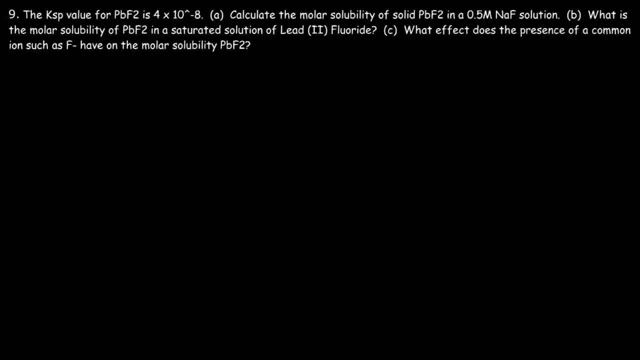 Multiplied by 811.54.. And so the solubility is now 5.04 times 10, to the negative 9 grams per liter. So that's the answer. Now let's focus on solving common ion effect problems. So in this problem we're given a Ksp value for lead-2-fluoride. 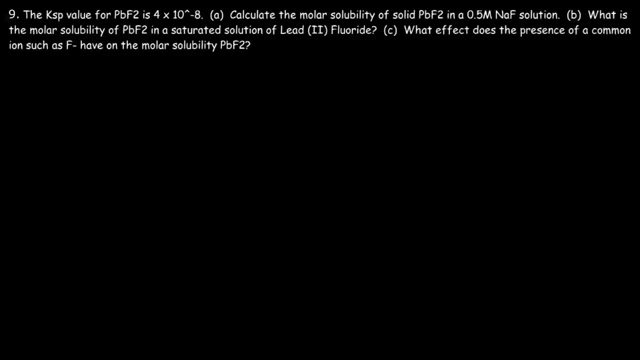 It's 4 times 10 to the negative 8.. And our goal is to calculate the molar solubility of solid PbF2 in a solution of sodium fluoride. So first let's write the dissolution reaction for lead-fluoride. 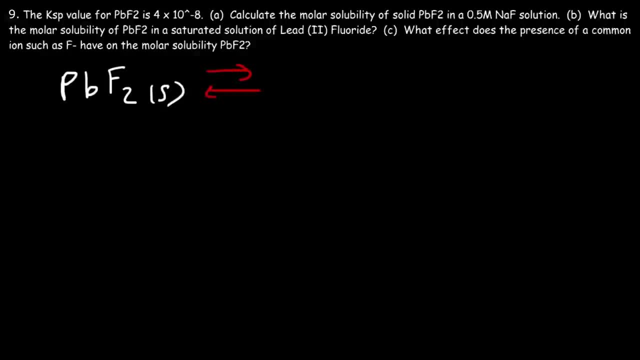 Lead-fluoride will dissociate into lead ions and fluoride ions. Now we need to balance the equation. So this is going to be 1, and then we need a 2 in front of fluoride. Now let's make an ice table. 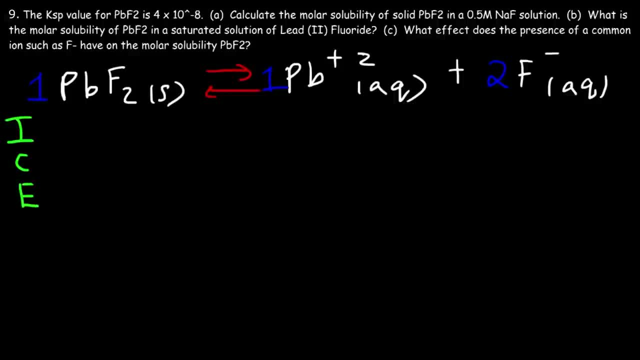 So initially the concentration of lead will be 0.. The concentration of fluoride is 0.5.. Because the lead-fluoride dissolves in a solution that already contains fluoride, Sodium fluoride is 0.5 moles per liter. 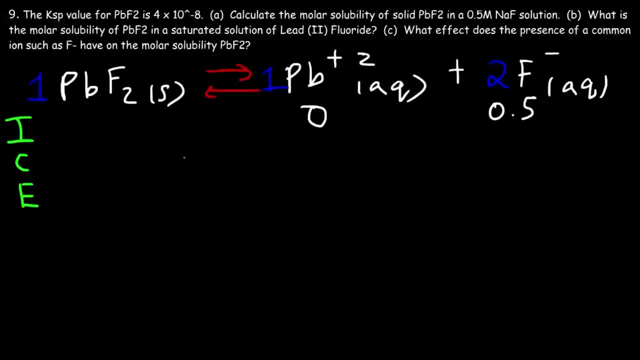 Now, because the concentration of lead is 0, the reaction has to shift to the right. So therefore, Pb will increase by x, or basically we could say 1x, And fluoride will increase by 2x, due to the 1 to 2 ratio that we see here. 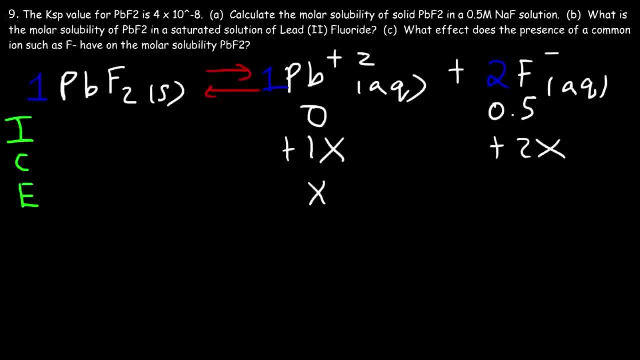 So in equilibrium the concentration of Pb plus 2 is represented by x And fluoride will be 0.5 plus 2x. So now let's write the Ksp expression. So Ksp is going to be product. So it's going to be products over reactants. 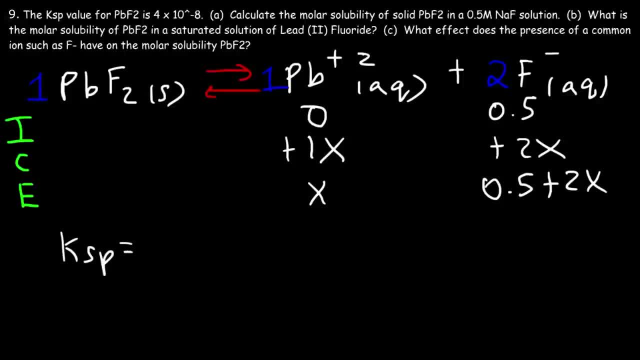 And the reactant is a solid, so we cannot include that in the equilibrium expression. So it's just going to be products divided by no reactants in this example. Now we need to raise this to the second power, So that's the Ksp expression for this reaction. 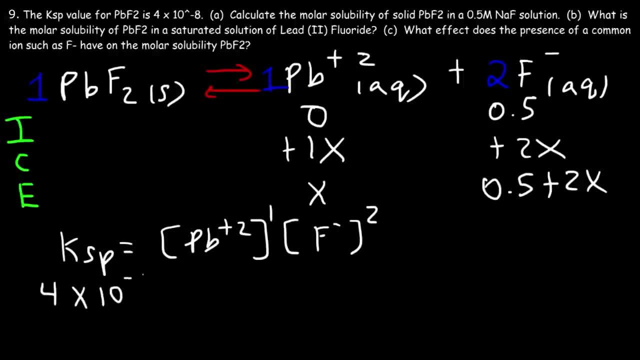 Now the Ksp is 4 times 10 to the negative 8.. And the concentration of the lead, 2 plus ion, we said we said it's x. And the concentration of fluoride is 0.5 plus 2x. 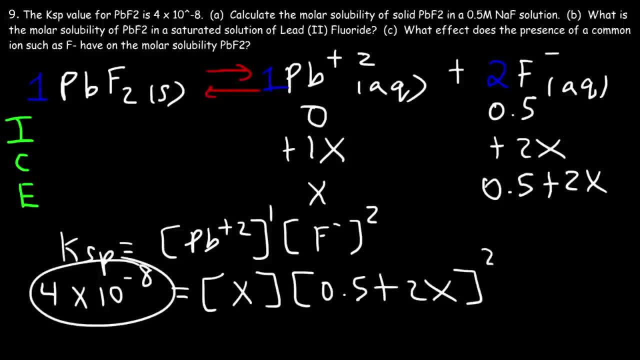 Now notice that Ksp is very small: 10 to the negative 8. That means x is going to be a very small value. So 0.5 plus 2 times a very small number is still going to be 0.5.. 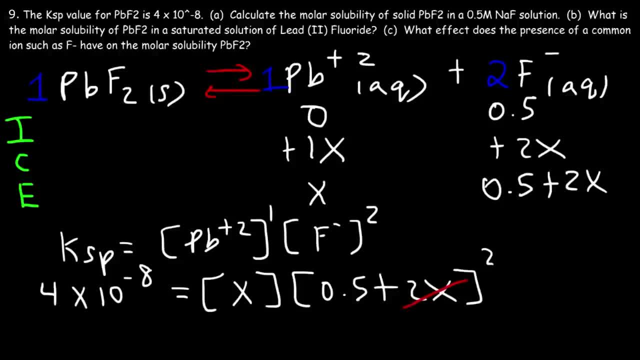 So this 2x quantity is negligible. So now we have this expression: 4 times 10 to the negative 8.. 4 times 10 to the negative 8.. 4 times 10 to the negative 8 is equal to x multiplied by 0.5 squared. 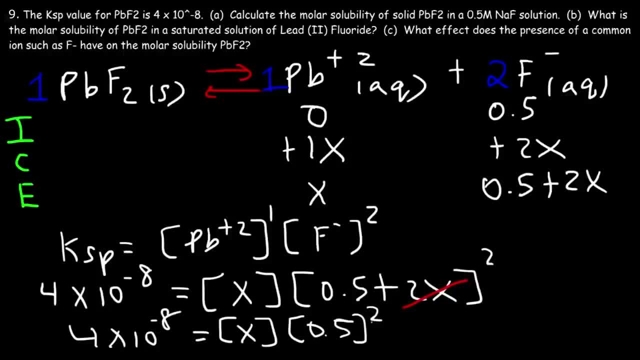 So to calculate the value of x, it's simply the Ksp value 4 times 10 to the negative 8, divided by 0.5 squared, And so x is equal to 1.6 times 10 to the minus 7.. 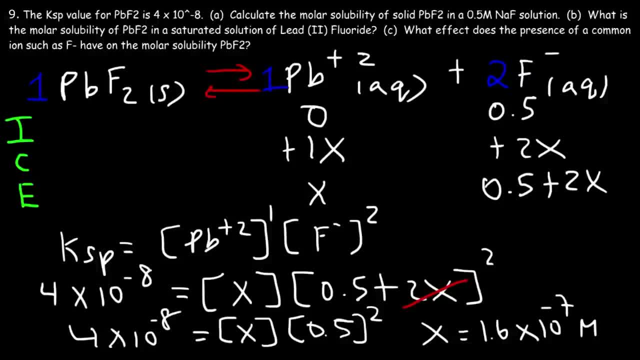 Now, x represents the concentration of the Pb plus 2 ion that's dissolved, And notice that the Pb plus 2 ion is in a 1 to 1 ratio with lead fluoride, So the amount of lead fluoride that's dissolved in the solution is equal to x in this example. 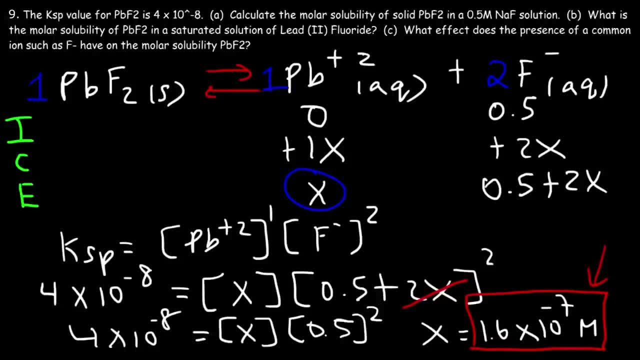 So x represents the molar solubility. So that's the molar solubility of lead fluoride in a solution of sodium fluoride. So that's the answer to part A. Now let's look at part B. Now let's focus on part B. 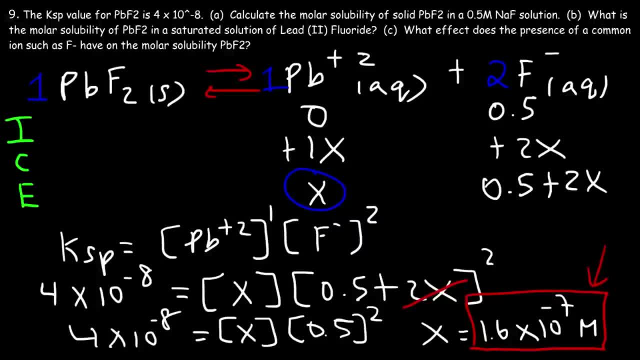 What is the molar solubility of lead fluoride in a saturated solution of lead fluoride? So in this example, we want to calculate the molar solubility. if it's not in a sodium fluoride solution, So it's just a solution that consists only of PbF2.. 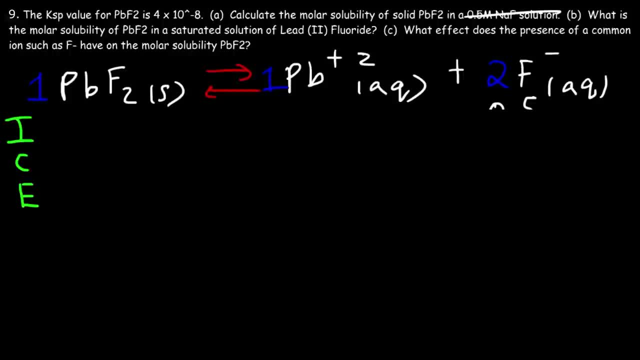 So how is this problem going to be different than the last problem? What would you say? In this problem, the concentration of lead is 0, but fluoride will be 0 as well. We don't have a common ion in part B. 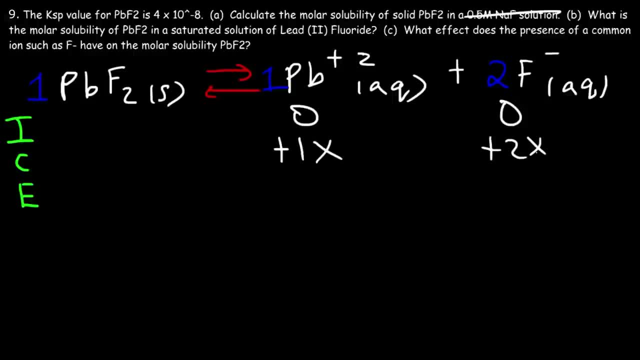 So this is going to increase by 1x. this will increase by 2x. So the Ksb expression, which is still going to be Pb plus 2 times the concentration of fluoride is squared. In this case, lead is still x, but fluoride is simply 2x. 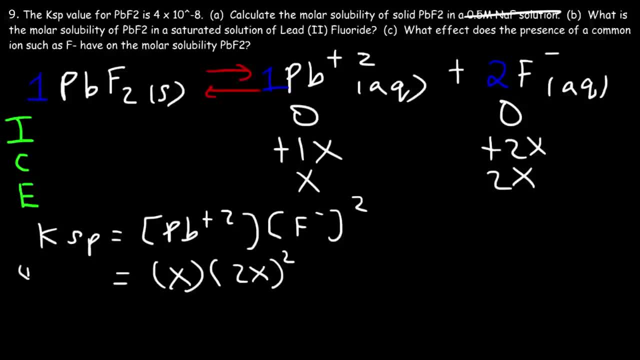 There's no 0.5 in this example, But Ksb is still going to be 4 times 10 to the minus 8.. Now 2x squared is equal to 4x squared, and 4x squared times x is 4x cubed. 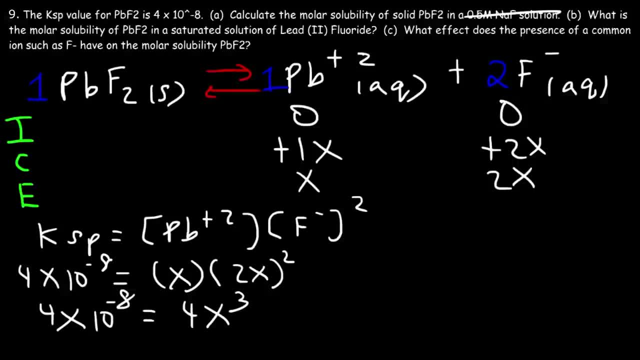 So our goal is to calculate x, which represents the molar solubility. Now keep in mind: for the previous answer, it was 1.6 times 10 to the minus 7.. Let's see what the new answer is going to be for part B. 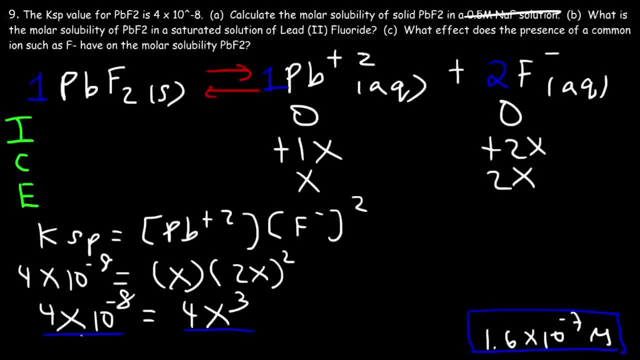 So first what we need to do is divide both sides by 4.. So 4 divided by 4 is 1.. So on the left side it's going to be 1 times 10 to the negative 8, and that's equal to x cubed.